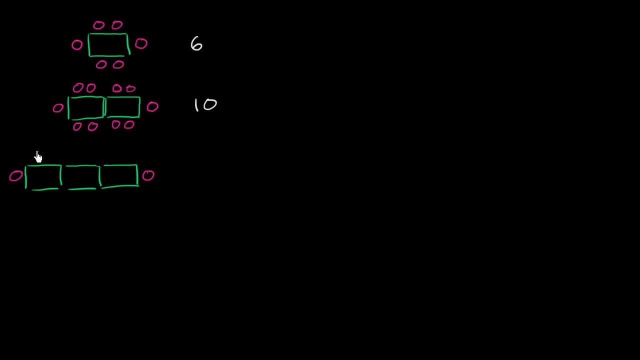 six, seven, eight, nine, 10,, 11,, 12,, 13,, 14 folks- 14 folks. So what does it look like is happening here? Well, if you just look at the numbers, we went from six to 10 to 14.. 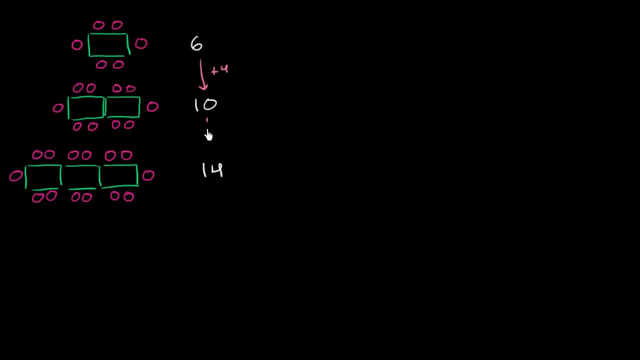 It looks like we're adding four people every time we actually add a table. Now does that actually make sense? So let's think. Let's think about this first situation. Let's imagine these are real people, And I'll make this person in blue right over here. 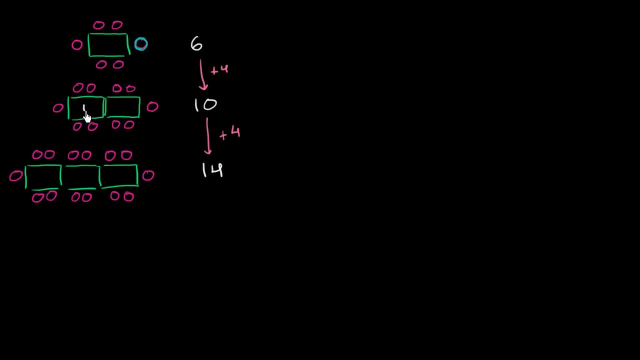 If you were to bring over this new table? if you bring over table two, so this is table one. If you bring over table two, this blue person has to move, And so where could they move? Let's say that they always insist on sitting. 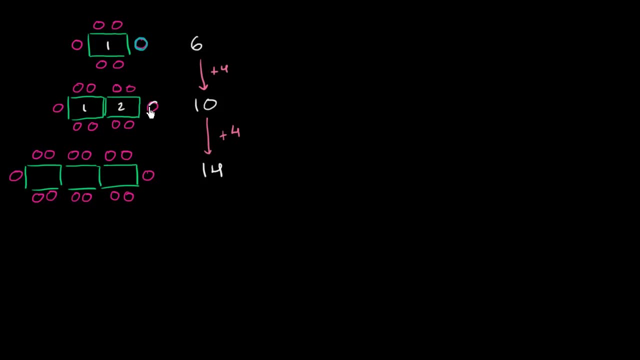 at the end of a table. So the blue person moves to the new end of the table. They move right over here. So how many new people could move to this combined table now that you brought the second table in? Well, the new people. I will do in this purple color. 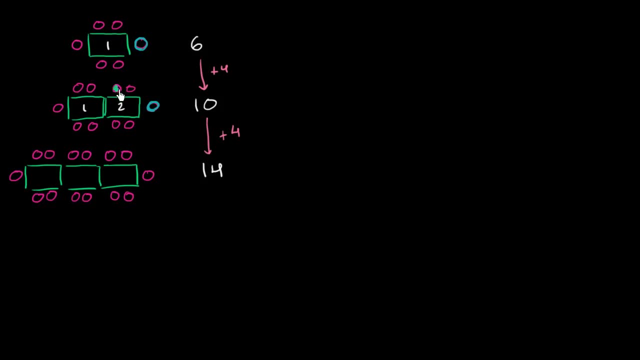 The new people are that person- Let me do it in a more unique color- This person, this person, this person and this person. So you were able to add four new people with a new table. One way to think about it is a new table. 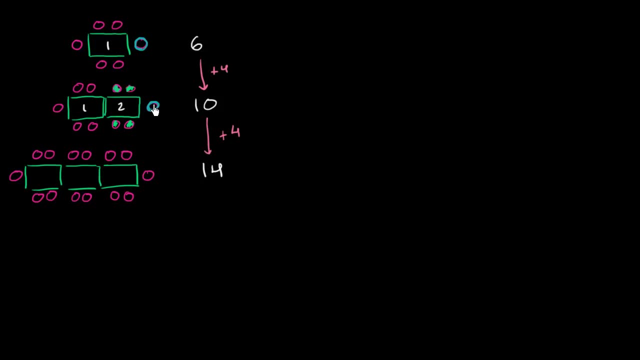 is going to have one usable end here. That usable end is going to be taken by the person who was already at the usable end of when you had less tables, And so you're really able to. the real addition is the two sides here. 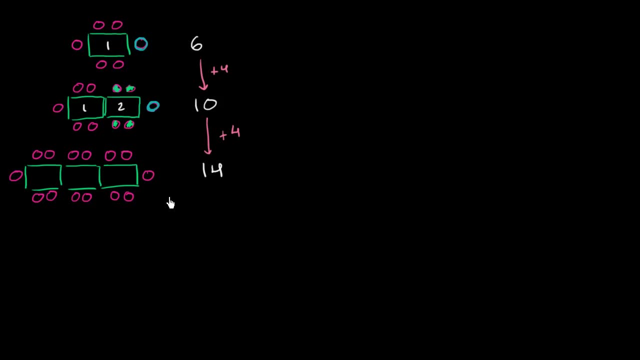 So you're adding four people every time you add a table, So it makes complete sense. So, based on this, you could think about, without even having to draw these diagrams, what would happen or how many people you would be able to fit if you had four or five or six. 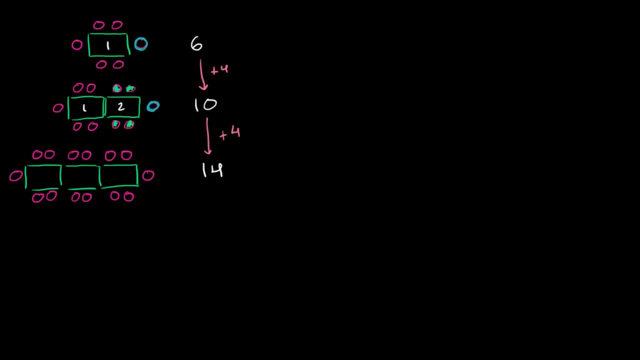 or however many tables. So you could imagine: if you have four tables, we just have to add four and you should be able to sit 18 people. If you have five tables, you should be able to fit 22 people, and on and on and on. 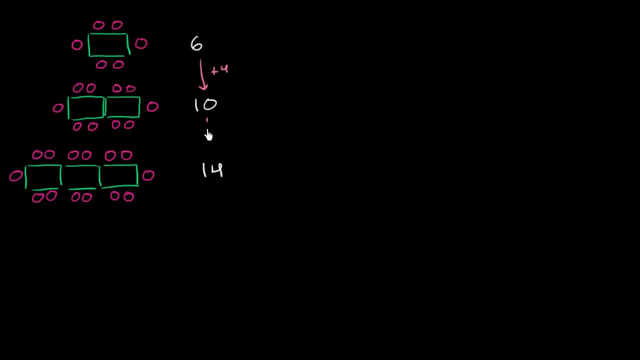 It looks like we're adding four people every time we actually add a table. Now does that actually make sense? So let's think. Let's think about this first situation. Let's imagine these are real people, And I'll make this person in blue right over here. 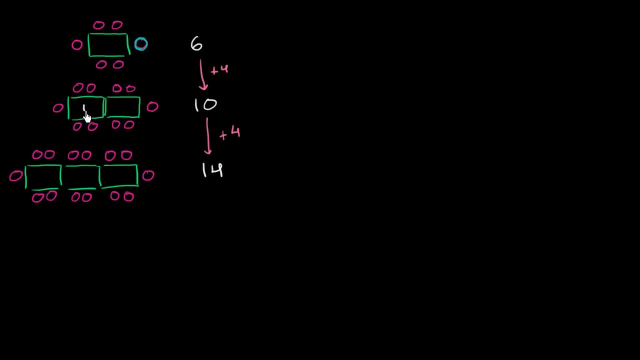 If you were to bring over this new table? if you bring over table two, so this is table one. If you bring over table two, this blue person has to move, And so where could they move? Let's say that they always insist on sitting. 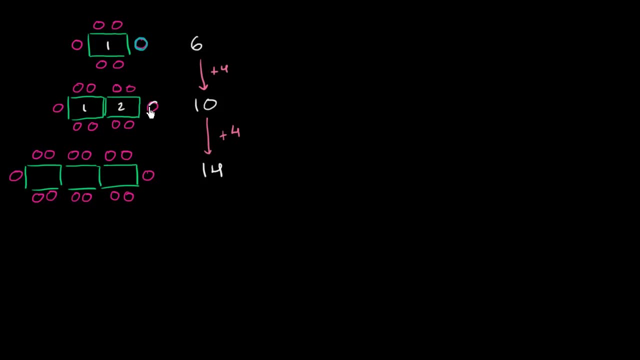 at the end of a table. So the blue person moves to the new end of the table. They move right over here. So how many new people could move to this combined table now that you brought the second table in? Well, the new people. I will do in this purple color. 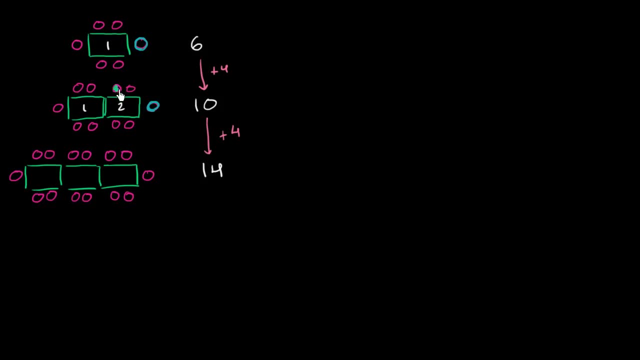 The new people are that person- Let me do it in a more unique color- This person, this person, this person and this person. So you were able to add four new people with a new table. One way to think about it is a new table. 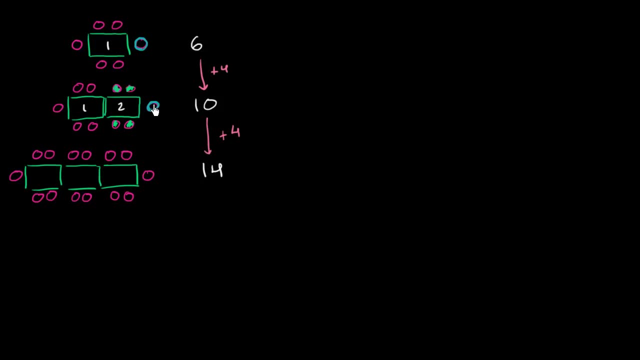 is going to have one usable end here. That usable end is going to be taken by the person who was already at the usable end of when you had less tables, And so you're really able to. the real addition is the two sides here. 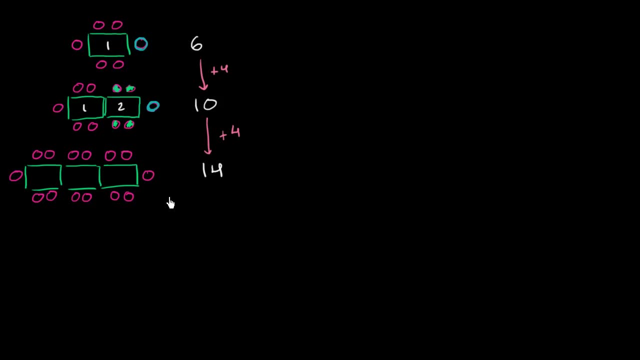 So you're adding four people every time you add a table, So it makes complete sense. So, based on this, you could think about, without even having to draw these diagrams, what would happen or how many people you would be able to fit if you had four or five or six. 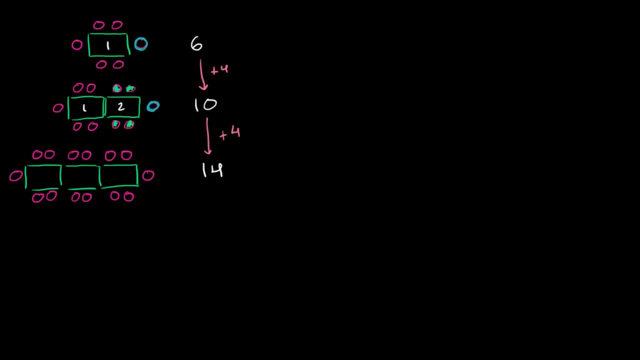 or however many tables. So you could imagine: if you have four tables, we just have to add four and you should be able to sit 18 people. If you have five tables, you should be able to fit 22 people, and on and on and on.